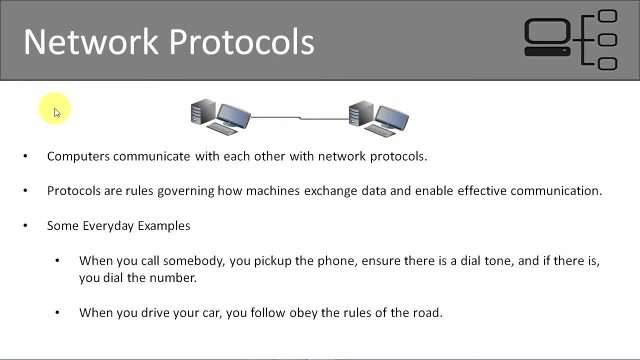 to really bring this to light and show it in a non-IT manner. Now another one is driving your car. So, just like calling on the phone, there are certain rules you have to follow, And when you're driving your car, there's rules of the road. You have to obey the speed. 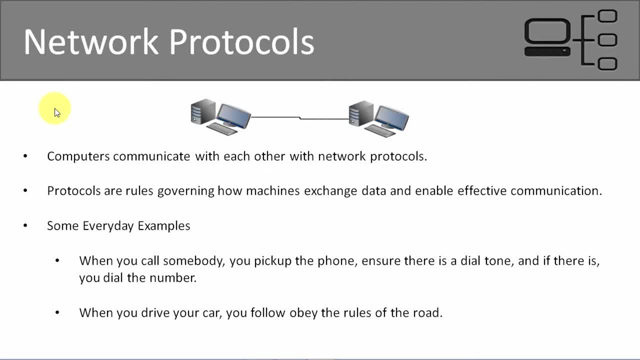 limit. You have to put your blinker on when you switch lanes And if you don't, then there's consequences. You can get a speeding ticket, You can get a ticket for driving improperly Or potentially you could even get in an accident. So when we are thinking about communication, 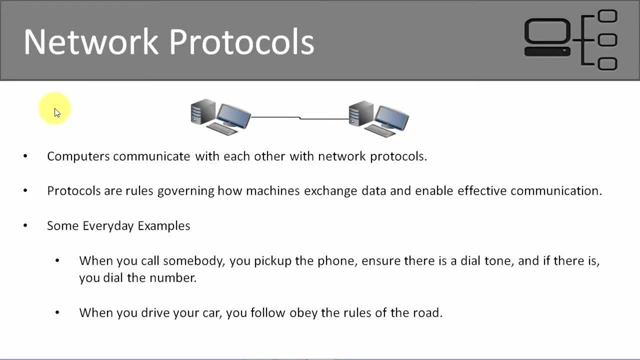 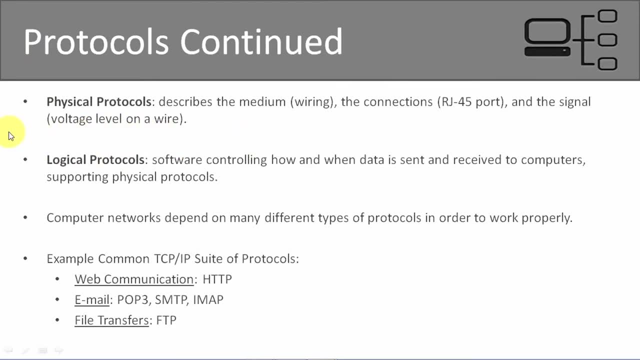 protocols or if we're thinking about protocols in general. just remember that those are rules and we have to follow those rules. So let's talk about these protocols in a bit more detail. Let's revisit our physical protocols and our logical protocols. So what is the physical protocol? Well, it's just like the. 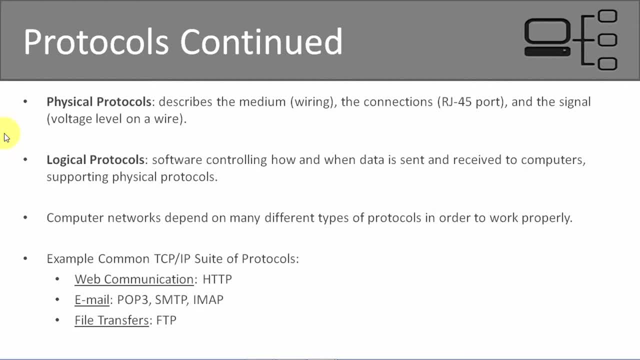 name implies It's the actual physical portion of the network. And so when we're thinking about, Let's talk about a network at its most simplest form, where we have two computers connected by one medium, one cable. Well, that actual cable with its connectors on the end and the 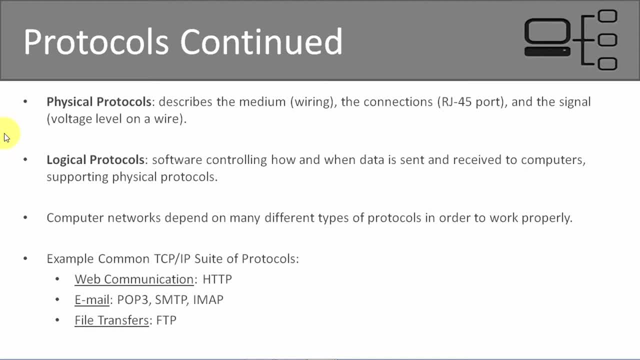 network interfaces that it plugs into. that's the physical protocols right there, And even the electrical signals that are going back and forth from one computer to the next. that's part of the physical protocol. Now, on the flip side, we have our logical protocols. 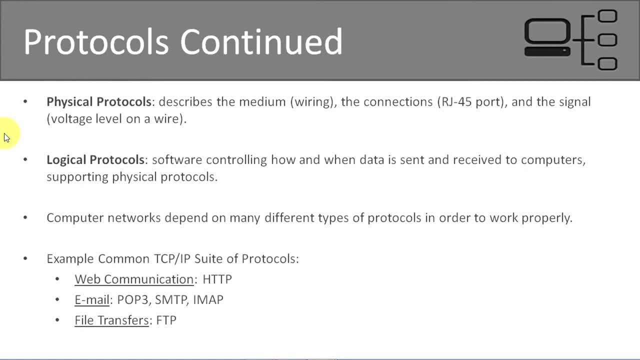 So the logical protocols is really how software controls how the data is sent and received And really how it's interpreted. So we have our machine code and we have all the other programming languages in place Where the software interprets it. it interprets the. 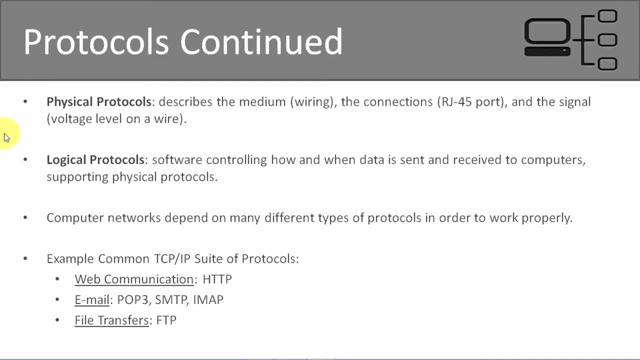 actual physical signal going back and forth And it interprets it as a logical protocol. Now, it's okay if you really don't understand this and it doesn't make that much sense. It's going to make a lot more sense as we go through the course. 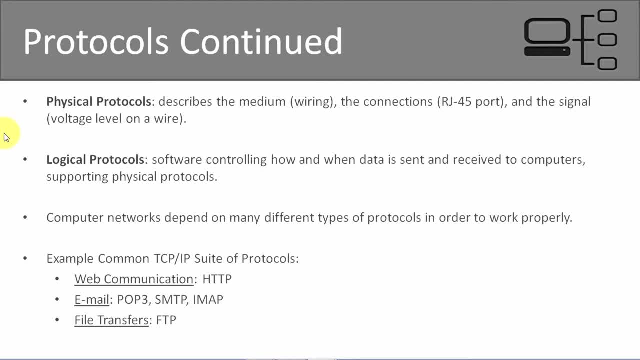 So in computer networks there's all sorts of different protocols, Physical protocols and logical protocols. you're conquered by the machine And so when you're in the scene you'll never recognize that this particular method makes sense. But if you know how to use the